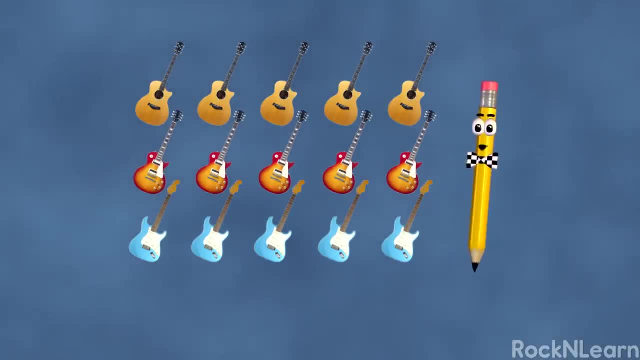 So, and that's where multiplication gives you power- What we actually have are one, two, three, four, five, groups of three guitars. Three, five times, or three times five equals fifteen. Notice that this sign means times, and it shows that you are multiplying. 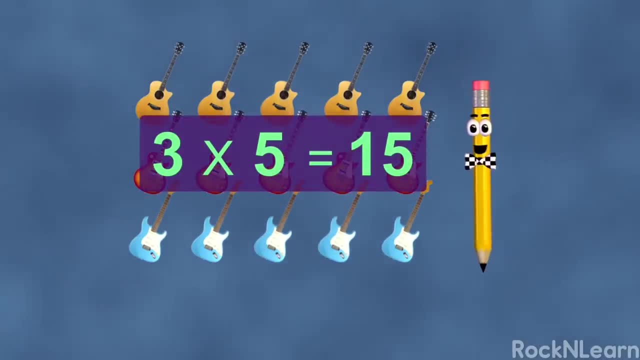 You can also write the problem this way: Three times five equals fifteen. So the power of multiplication is that it takes something slow, like adding the threes one set at a time And bada-bing: It makes the process faster in one step. 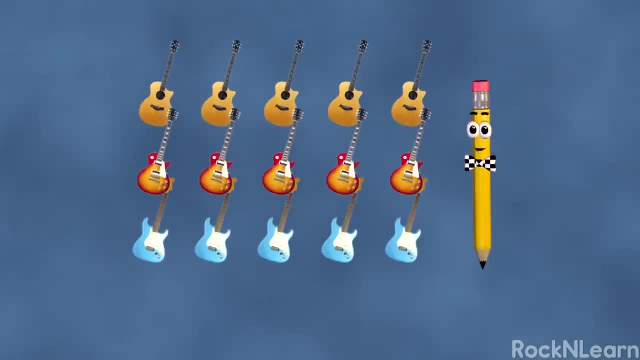 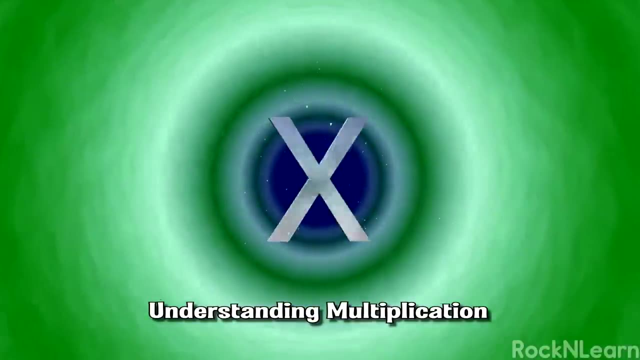 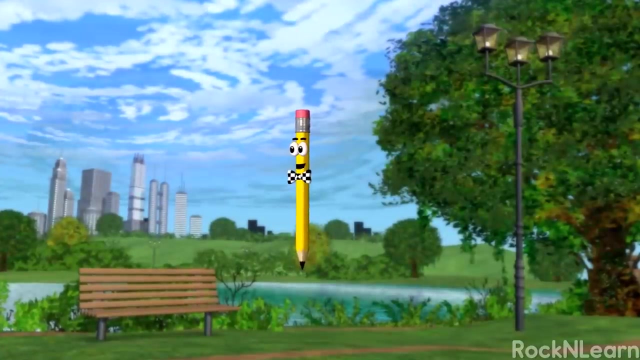 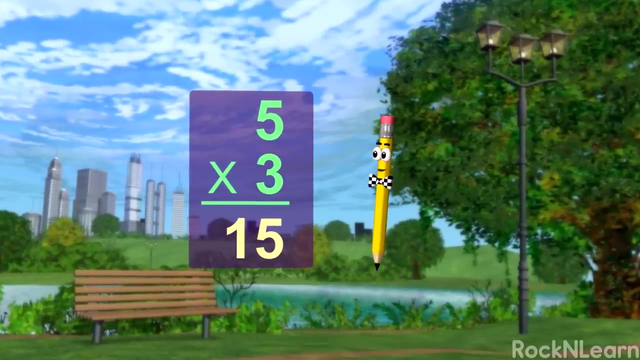 Are you getting the power of multiplication Loud and clear, Magnifico. Now, the numbers in a multiplication are like this: What? The numbers in a multiplication problem have special names. The numbers we are multiplying are called factors And the answer is called the product. 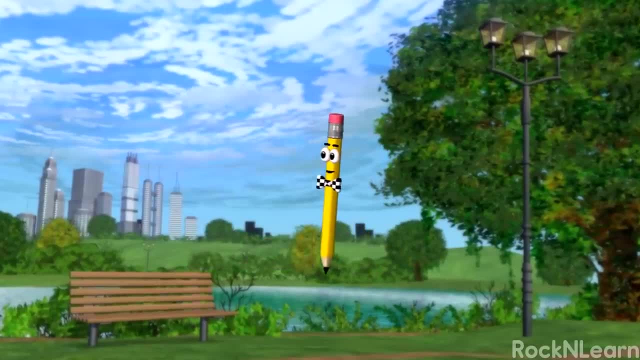 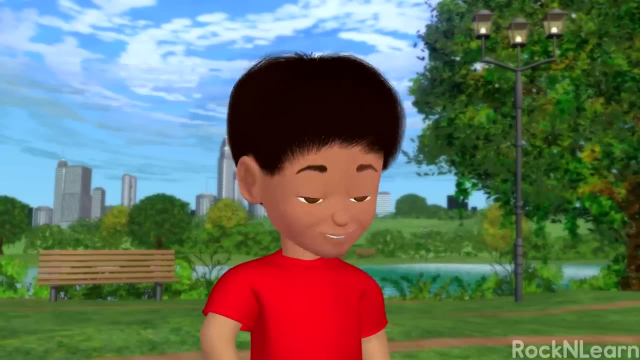 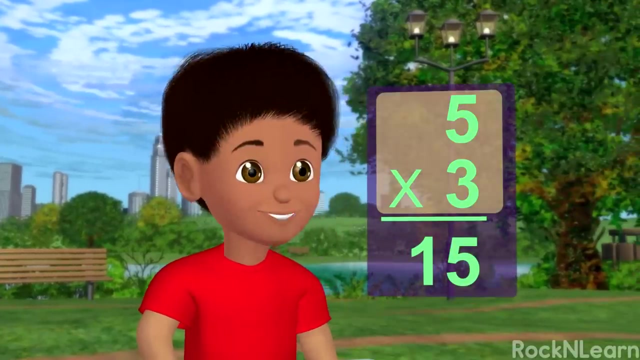 You can remember this quite easily because you go to stores to buy products, right, And where are those products? often made? Factories. That sounds kind of like factors. Oh, you're good, You, you're good. So we multiply the factors in this factory. part of the equation. 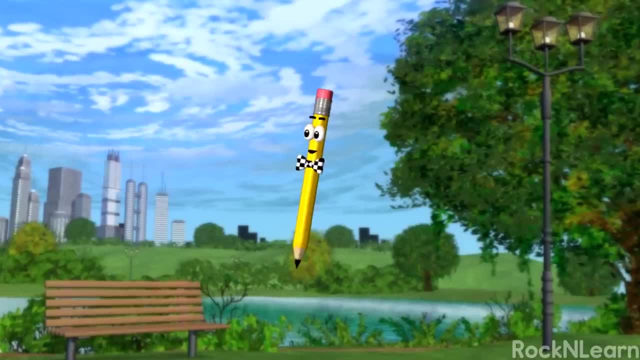 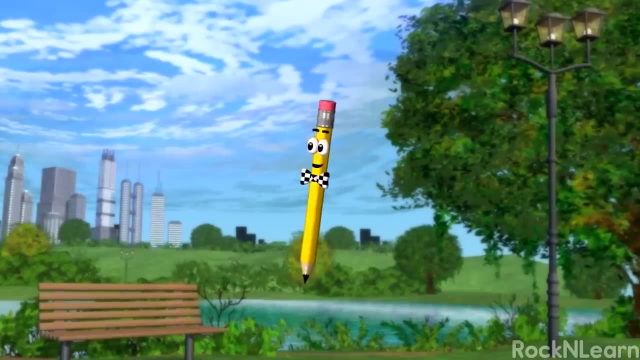 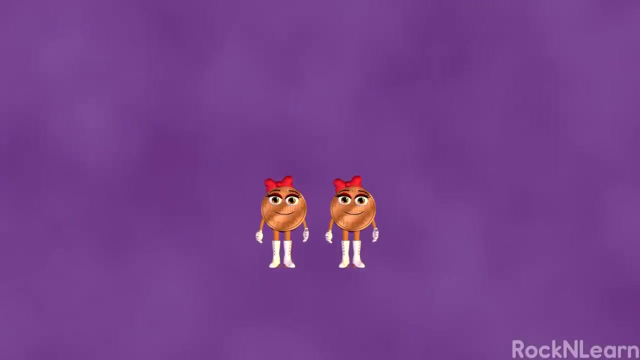 to get our product or answer. Smart boy, I like it the way you think. Now I know a great way to practice multiplication and really experience what it's all about. I'm going to need some pennies. Did somebody call for us? 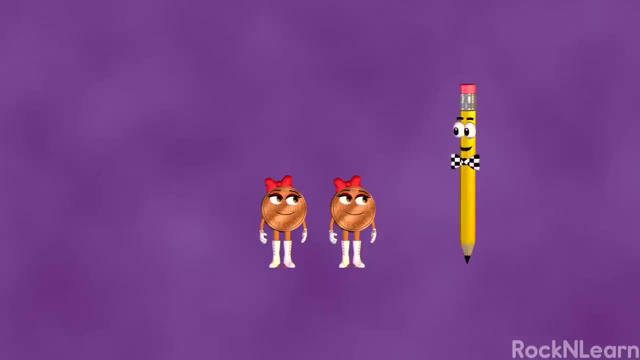 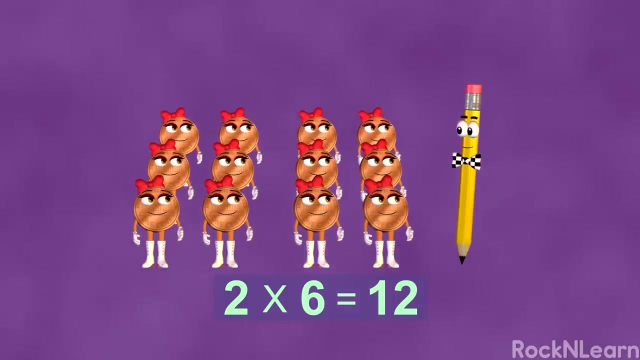 Actually, yes, but I need even more pennies. So how many of us do you need? Could I perhaps get twelve pennies? Okay, we'll just multiply ourselves times six. Is this better? Certainly, Two times six is twelve. 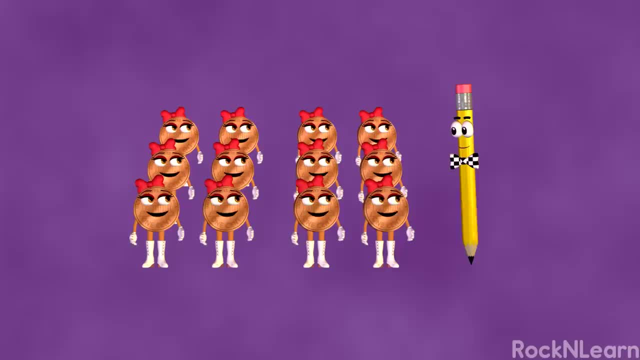 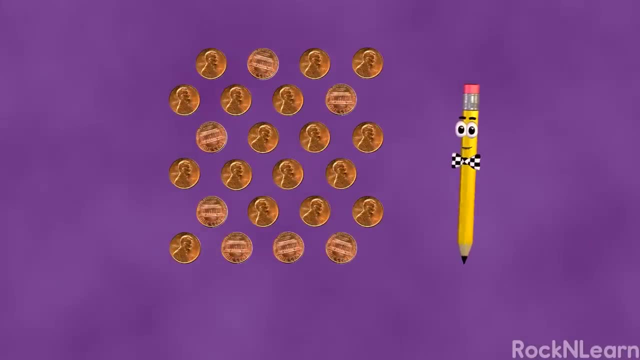 But I was hoping to get some real pennies. We're not real, Oh no, This is terrible. My pennies, Let's work with these real pennies. You can get your own pennies and easily practice this yourself. Take six groups of four pennies. 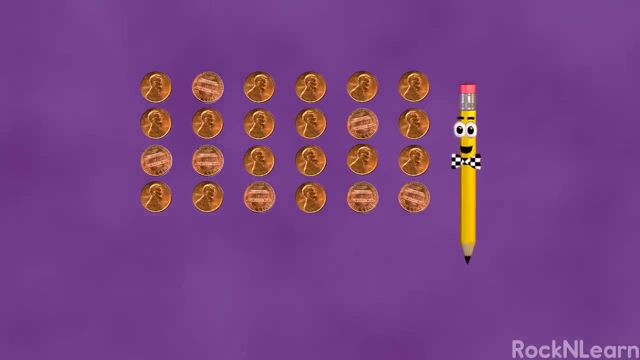 To know how many pennies you have. you could count them: One, two, three, four, five, six, seven, eight, nine, ten, eleven, twelve, thirteen, fourteen, fifteen, sixteen, seventeen, eighteen, nineteen, twenty, twenty-one, twenty-two, twenty-three, twenty-four. 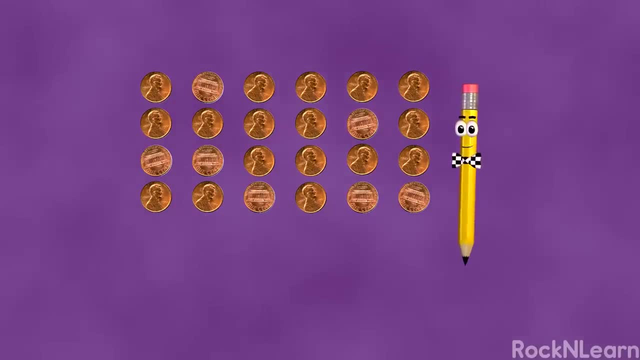 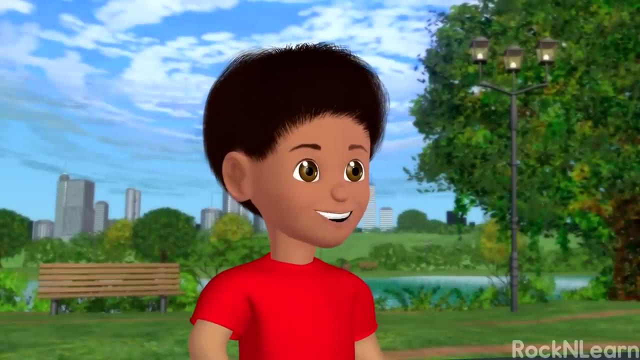 But if you know your multiplication facts, a much easier way is to say: Four times six equals twenty-four. That is much better. Now I know why it's important to learn my multiplication facts. It can save me a lot of time in the long run. 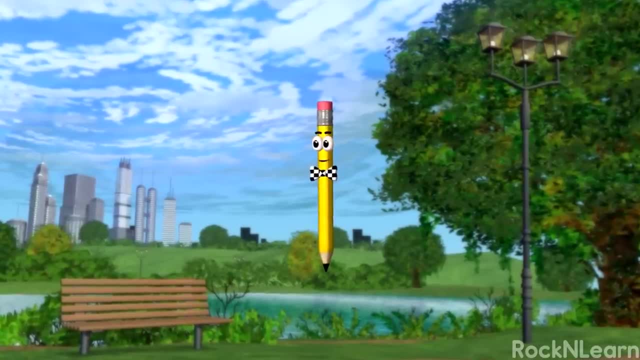 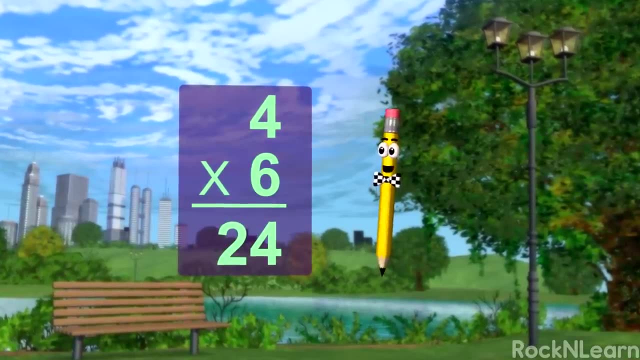 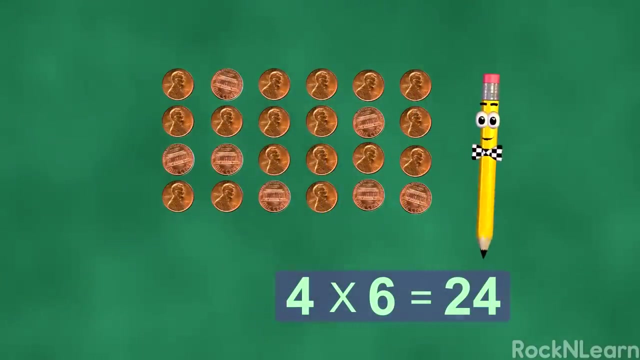 Right. Another great thing about multiplication is that the order in which you multiply the factors does not matter. We can change the order of the factors and, presto digio, The product does not change. Let me show you why. This shows the matrix. 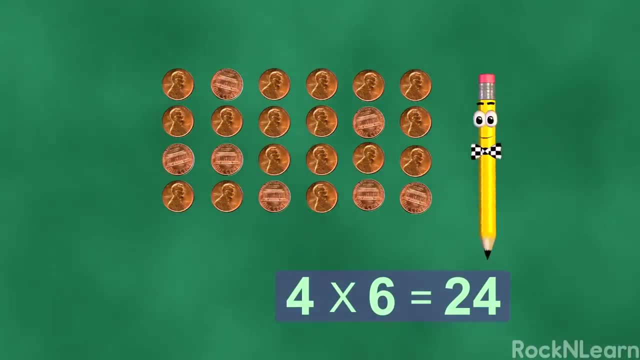 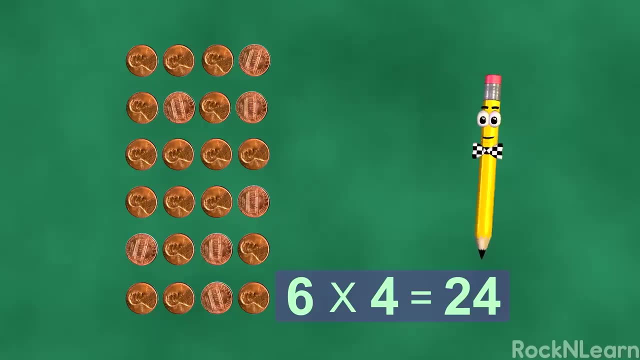 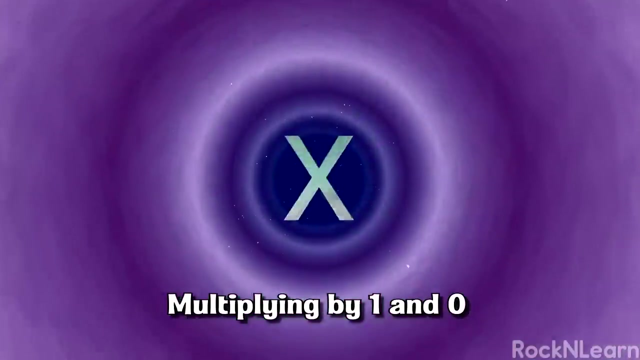 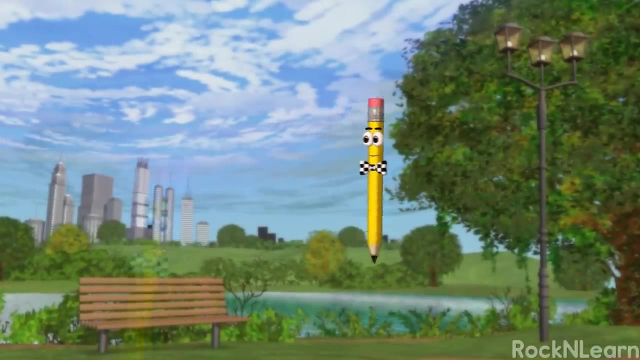 It shows the multiplication problem four times six. And if we move it around like so, it now shows the multiplication problem six times four, But we still have the same number of pennies, twenty-four. Oh, I understand. Let me show you some other neat tricks with multiplication. 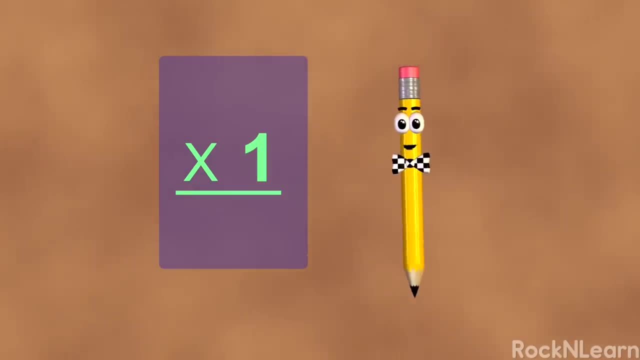 When you multiply a number by one, the answer is always that same number. Four times one equals four. Six times one equals six. Eight times one equals eight. Fifty times one equals- you guessed it- fifty. That's easy to understand. 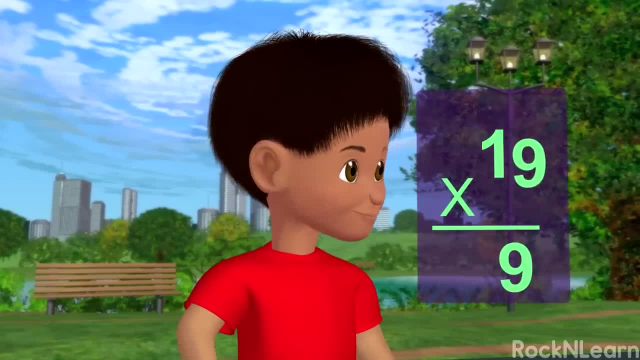 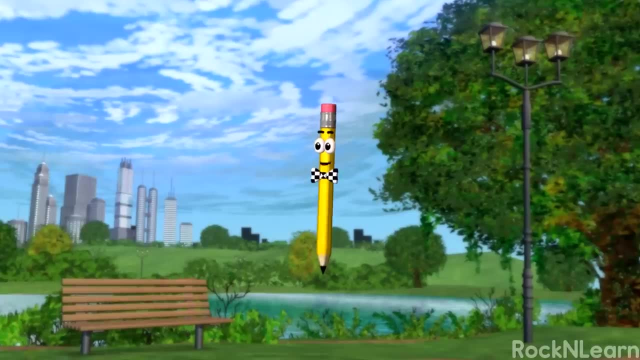 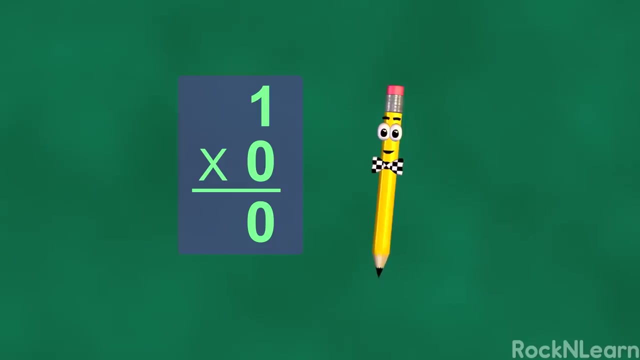 And since you can switch the places of the factors, I'll bet you can multiply one times any number and your answer will always be that number. That's right, You're bright. Here's another trick: When you multiply by zero, you always get zero. 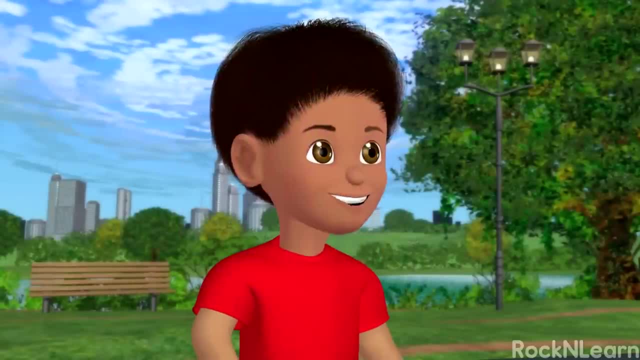 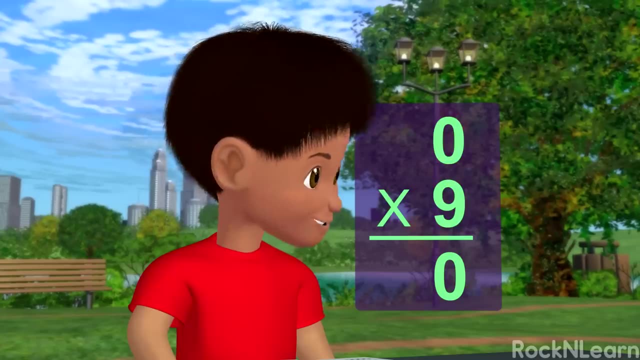 Any number times zero always equals zero. That just makes sense, Marco. If you have zero groups of something, you don't have anything, And if you swap that around, no matter how many times you add zero to zero, you'll always get zero. 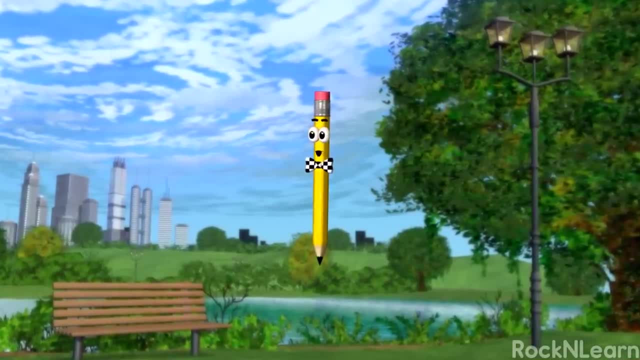 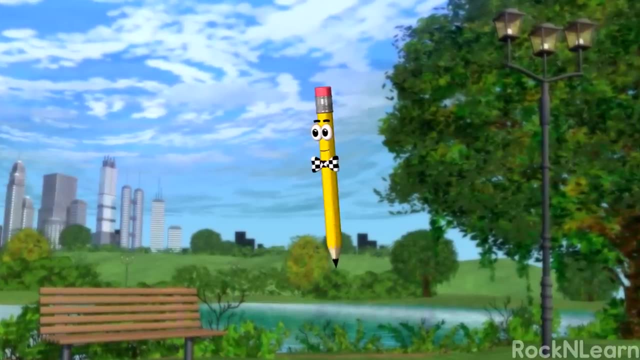 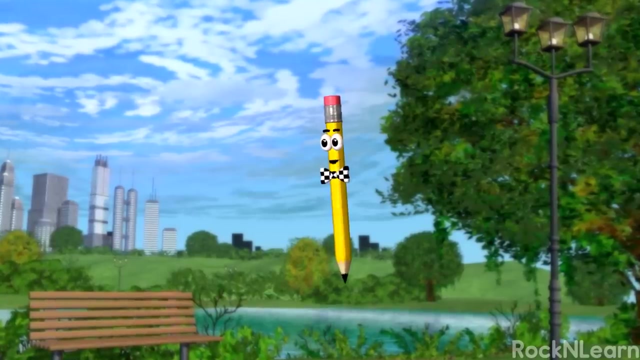 Perfecto. Now how do people get good at multiplying? Uh, they could use a calculator. Well, it's not always convenient to use a calculator. Smart people- and smart pencils for that matter- memorize their basic multiplication facts from one times one all the way up to nine times nine. 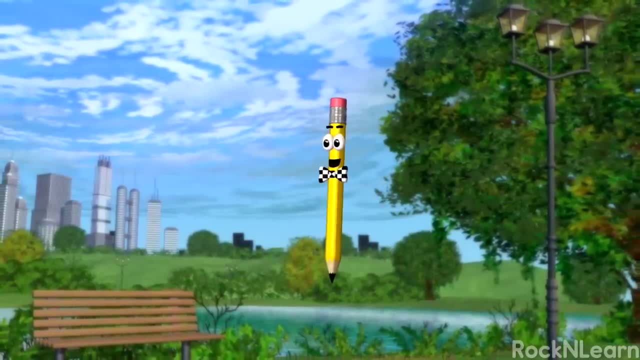 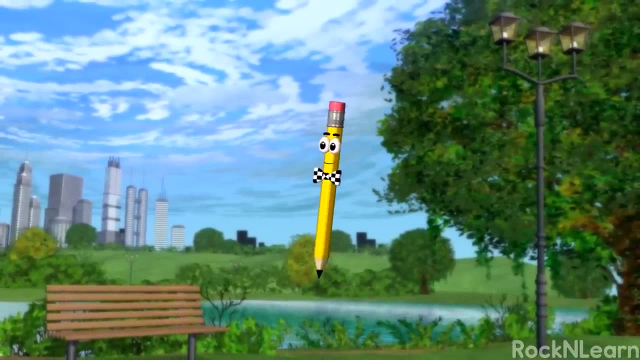 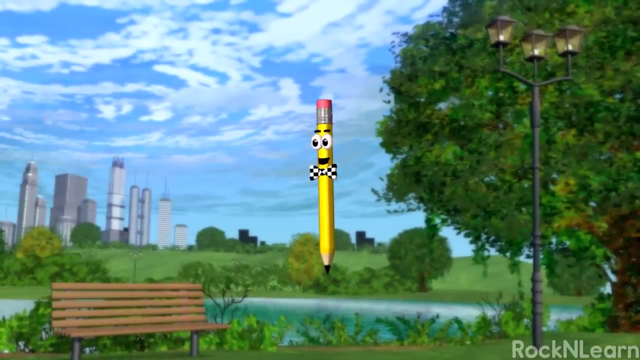 Some people even like to memorize all the way through the twelves. How am I gonna do that, Marco? The same way you get to Carnegie Hall kid Practice? Huh, Never mind. One easy way to memorize your multiplication facts is with a beat. 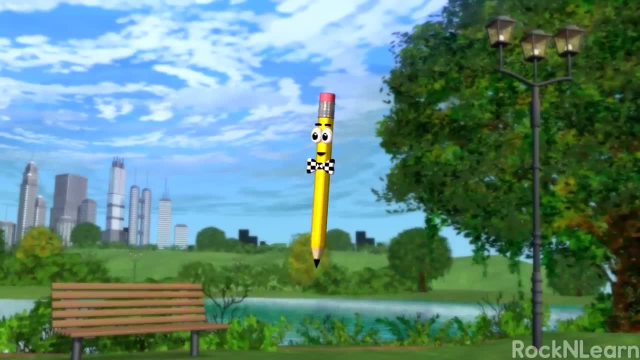 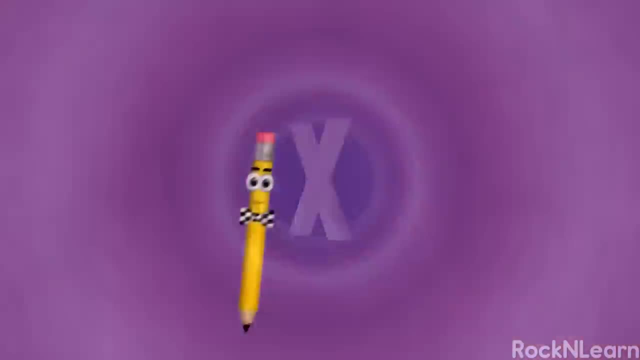 You can also practice skip counting. Whatever you do, practice makes perfect. I want to show you a trick that you can use to help you learn multiplying by nine. Can you give me a hand? I don't seem to have any at the moment. 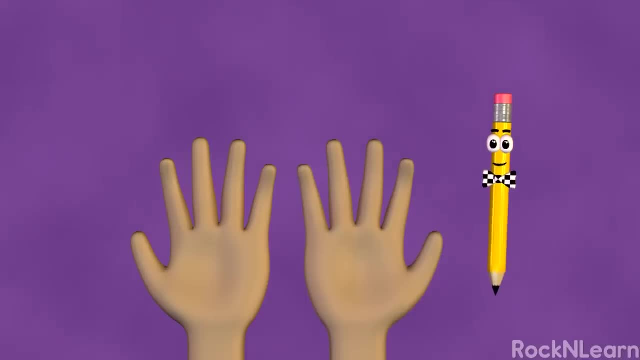 Actually I need two hands To multiply any number by nine. look at your ten fingers, palms facing you. Your fingers are numbered this way: Count from the left until you reach the number you want to multiply by nine and bend down that finger. 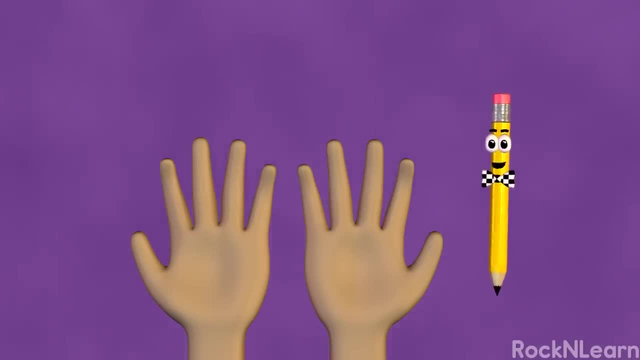 Count the fingers to the left of the bent finger for the number that goes in the tens place. The fingers to the right of the bent finger give you the number in the ones place. For example, to calculate three times nine, bend down the third finger. 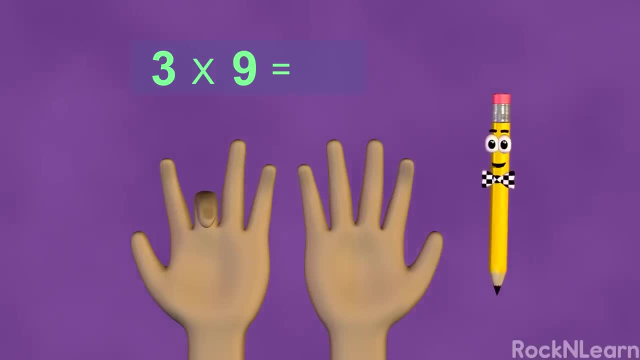 There are two fingers to the left of the bend and seven fingers to the right, So the answer is twenty-seven. To find the answer to four times nine, bend down the fourth finger. There are three fingers to the left of the bend and six fingers to the right. 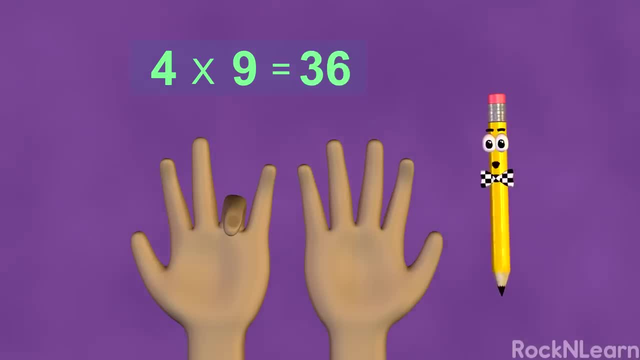 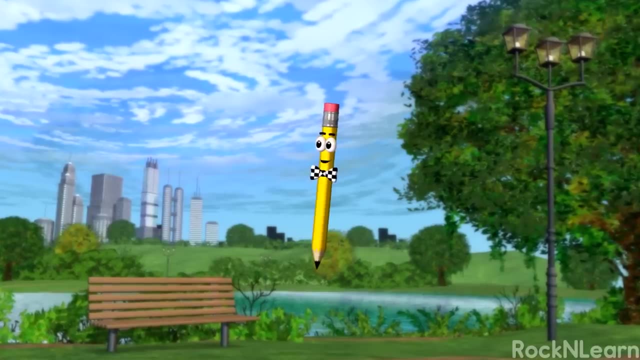 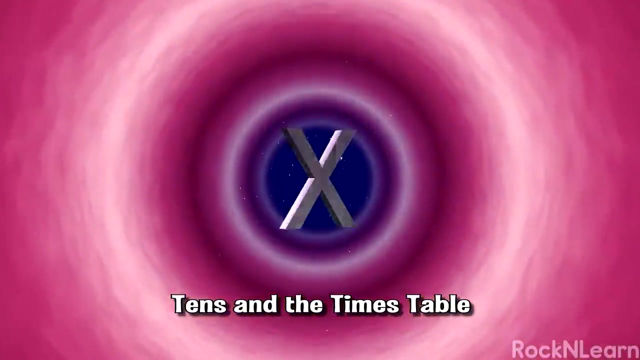 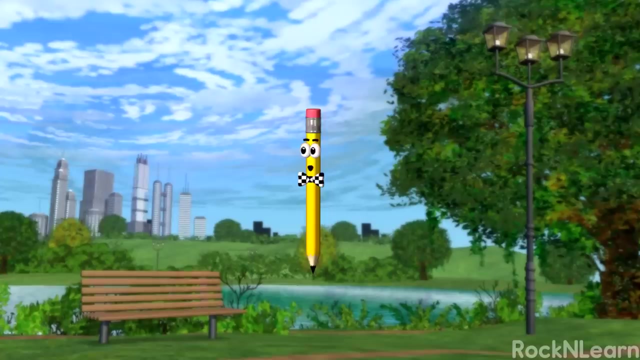 Four times nine is thirty-six. Wow, I love that trick. It only works when multiplying by the nines, but you must admit it's pretty handy. Hey, Marco, can you show me some more tricks? No, Please, Okey-dokey.